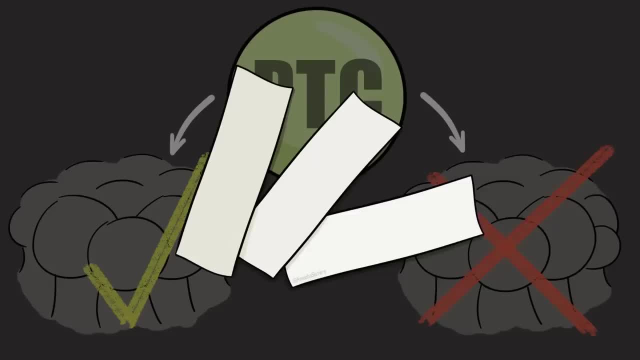 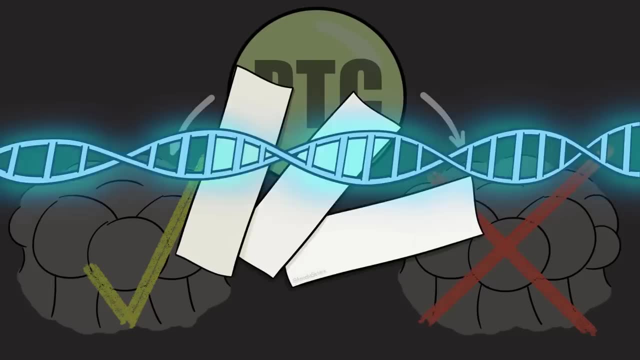 I guess I'll never know for myself what it would have tasted like. Of course, the reason PTC paper is used in genetic classes is because the trait of being able or not being able to taste PTC is based on genetics. A reminder from our Intro to Heredity unit. 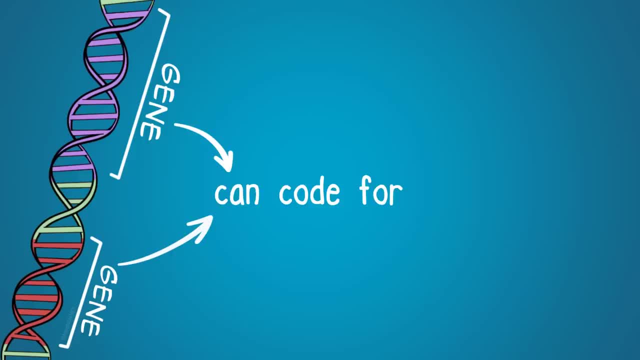 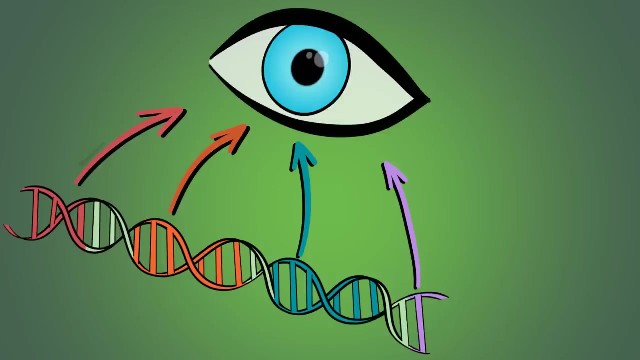 that genes are portions of DNA and they have the ability to code for a characteristic, a trait, like being able to taste or not to taste, PTC. Now we do want to point out that many traits are actually coded for by interactions of more than one gene, like eye color, which 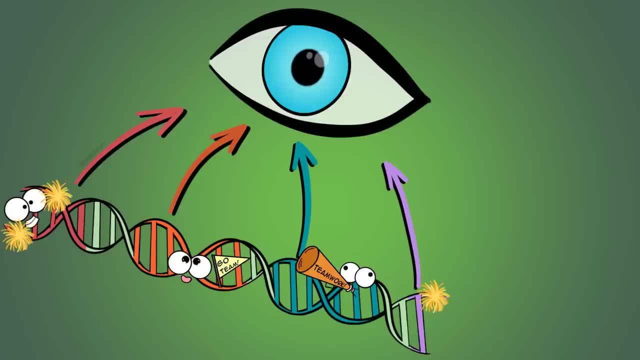 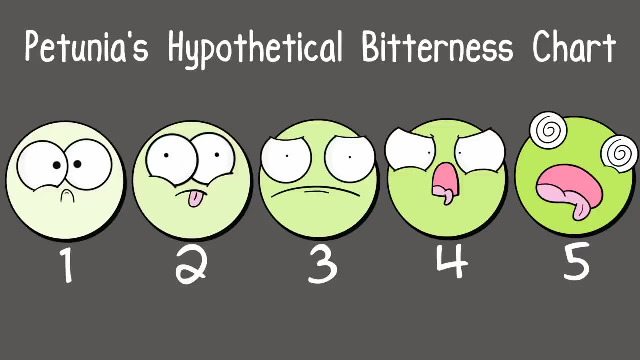 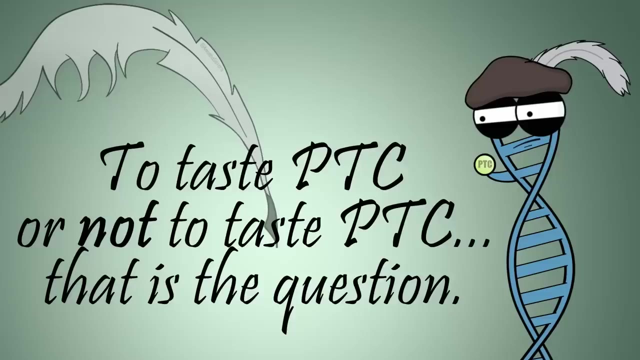 is quite complex and determined by interactions of many genes together. In fact, the ability to taste PTC or not may involve some other gene interactions. There's even different ranges for how bitter the chemical may taste, because there may be more kinds of alleles than we'll mention. More about that later. But since we do know that the ability to taste 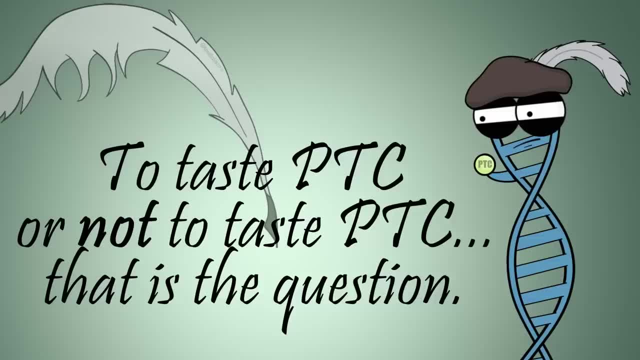 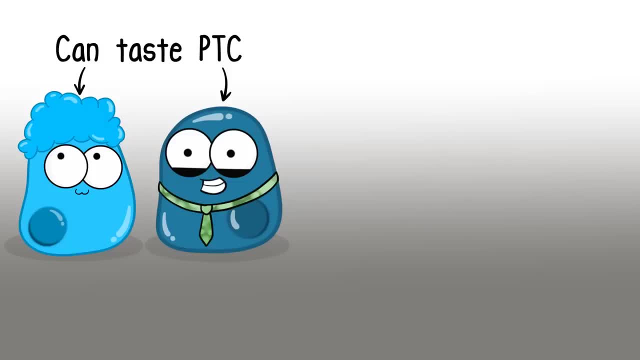 PTC or not taste PTC is at least heavily impacted by a specific gene. it does make it powerful for genetic classes. One thing I have found so interesting about this paper is that it's very clear that my parents can both taste PTC, So why can't I Recall that humans? 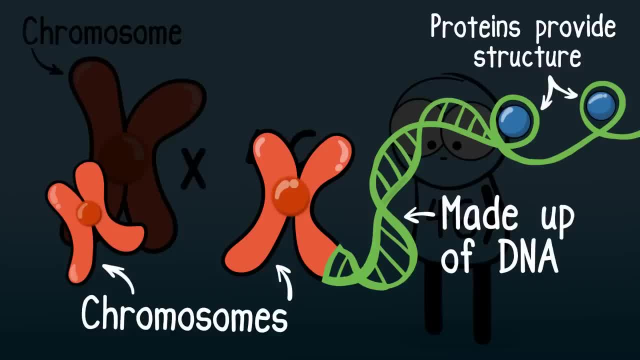 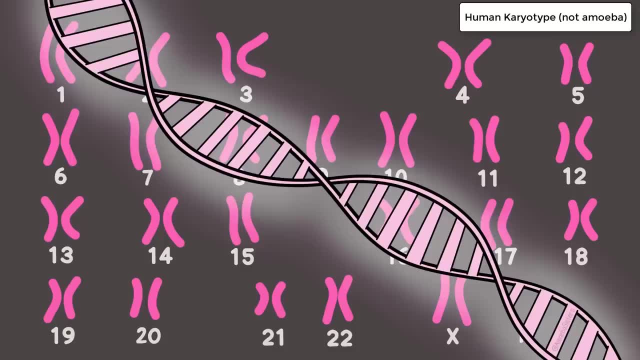 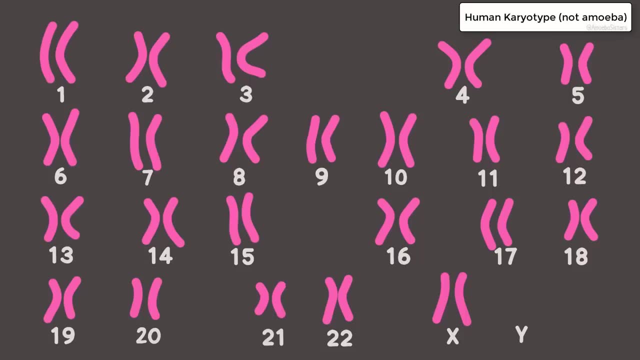 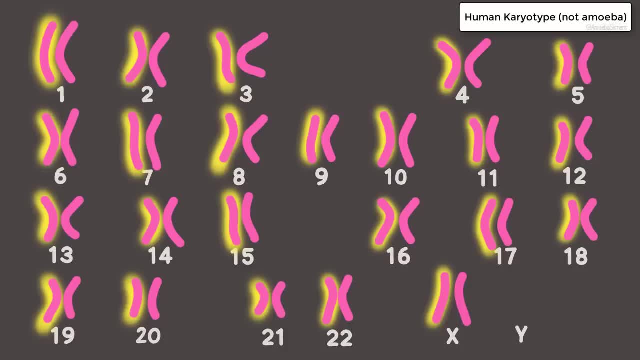 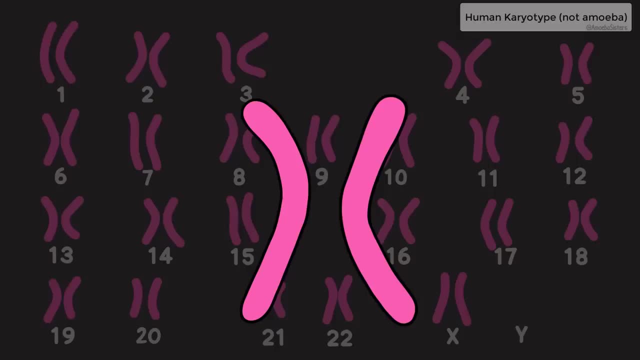 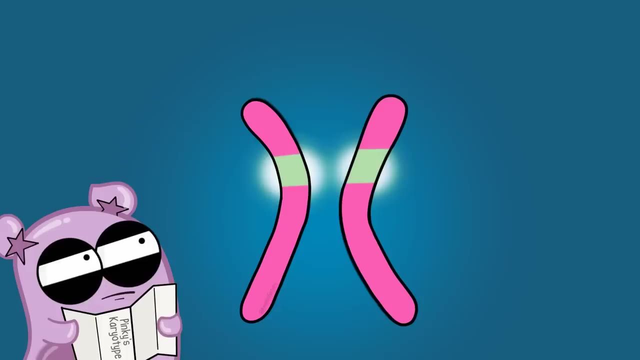 seeing this. Each pair has one chromosome from one parent and one chromosome from my other parent. If we focus on one of these pairs of chromosomes where the PTC taste sensitivity gene may be found, we can see an area where the PTC taste sensitivity gene could be. Let's 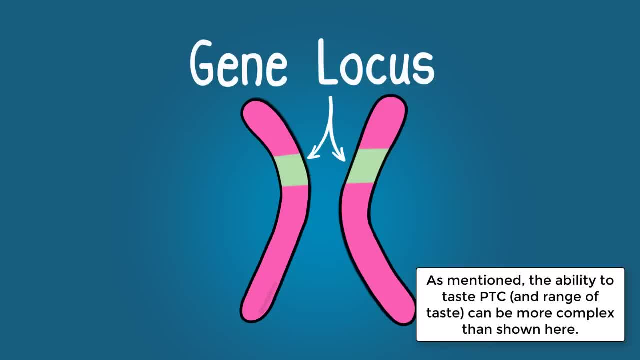 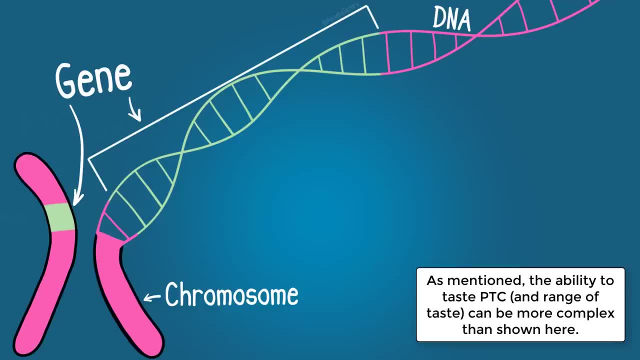 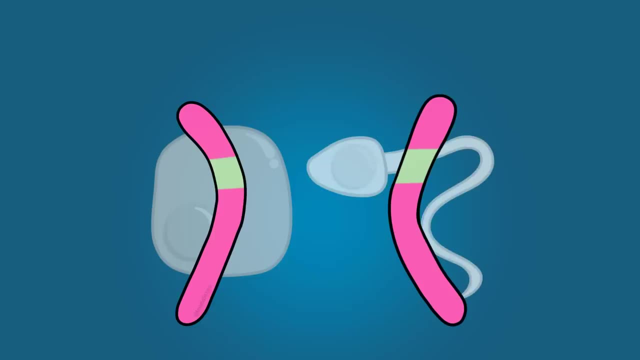 assume this is the locus where the PTC taste sensitivity gene is found. See how it is pointing to a specific area here. That's because it's on an area of the chromosomes that refer to a specific gene that codes for a trait. Now remember how. this chromosome is from mom, This one is from dad. Each parent contributes. 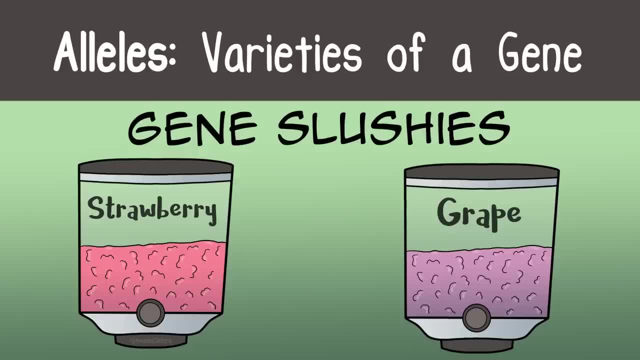 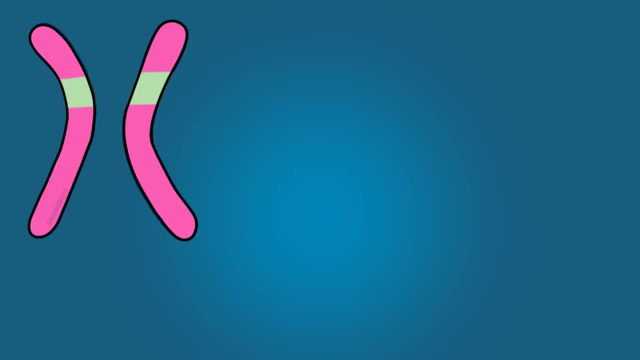 an allele, which is a variant of a gene. An allele is a variety of a gene, a form of a gene. The alleles could be the same form of the gene or different forms of the gene, but regardless, in this case, they're forms of the gene involved with PTC: taste sensitivity. 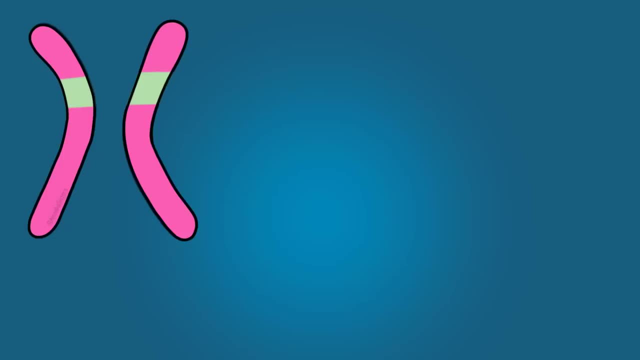 So if PTC taste sensitivity is being used as a one-to-one relationship between the two- one gene trait example- and as we mentioned, it may not be that simple- then your DNA code has a gene related to PTC taste sensitivity. Together the two alleles you inherit, the 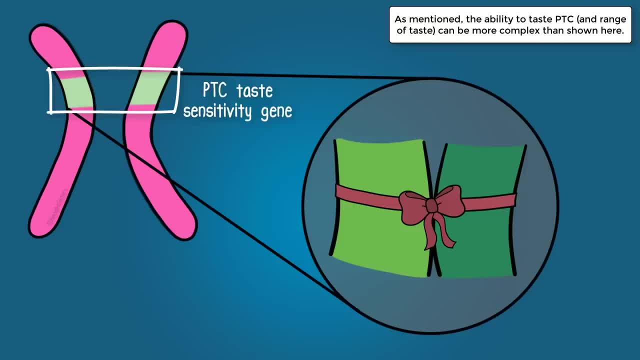 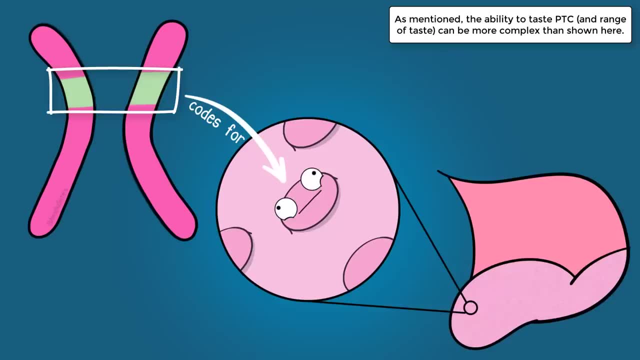 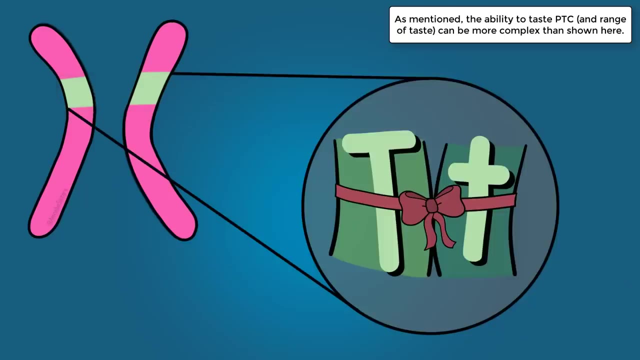 forms of that gene determine the trait of tasting PTC or the trait of not tasting PTC. That gene is involved with coding for taste receptors on your tongue and the receptors you have can make a difference for whether you taste PTC or not. The alleles are typically: 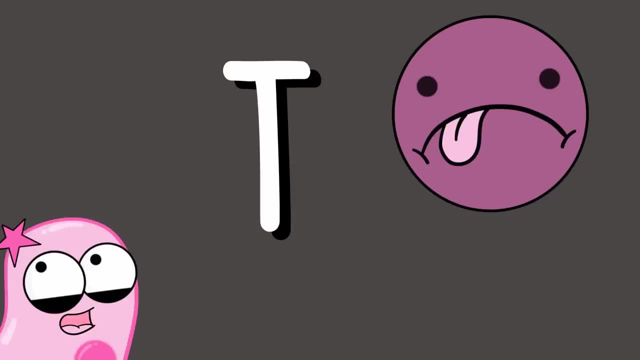 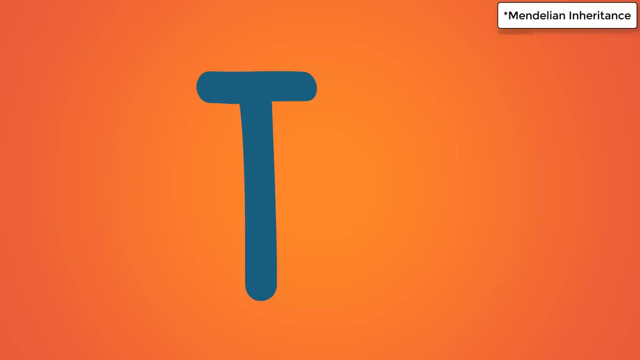 represented by letters. Since this is all about tasting, let's use the letter T. But wait, it matters whether I represent it as a capital or lowercase letter. If I use a capital letter to represent an allele, it means that it's a dominant allele, If one. 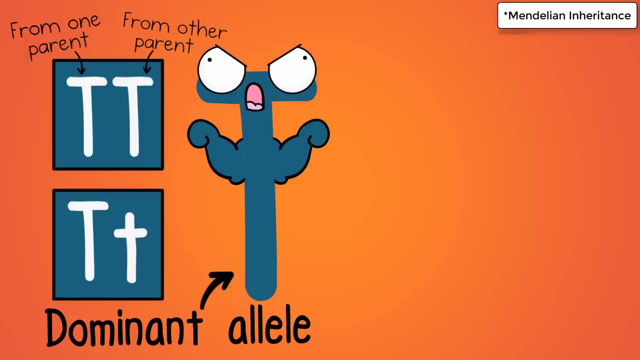 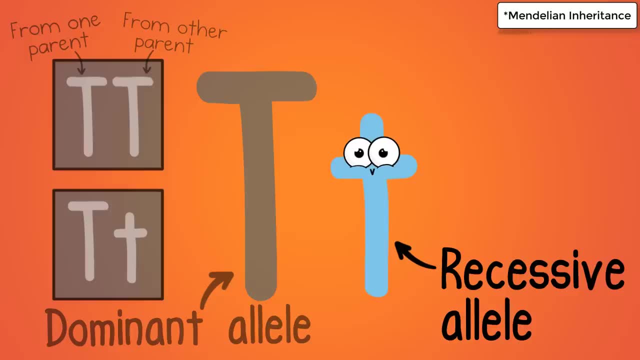 or both of the alleles you inherit for a trait are dominant, then it will be expressed More about that later. If I use a lowercase letter to represent an allele, that means it's a recessive allele. Recessive alleles are typically not expressed unless there is no dominant allele present. 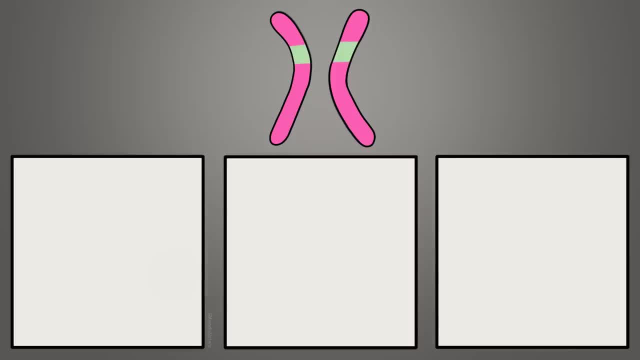 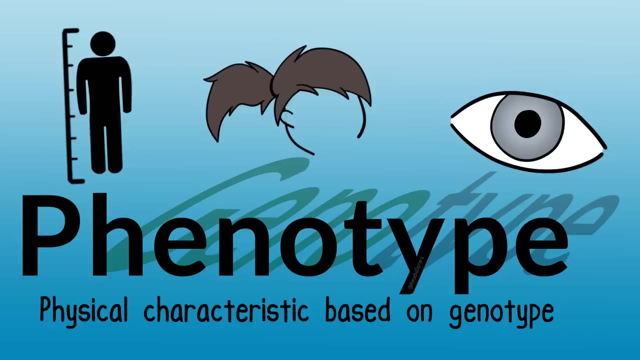 Now remember that you have two allele copies, so the combination you could have here could be big T, big T, big T, little t or little t, little t. These are called genotypes, your genetic makeup. Genotypes can help determine a phenotype, which is a physical characteristic. 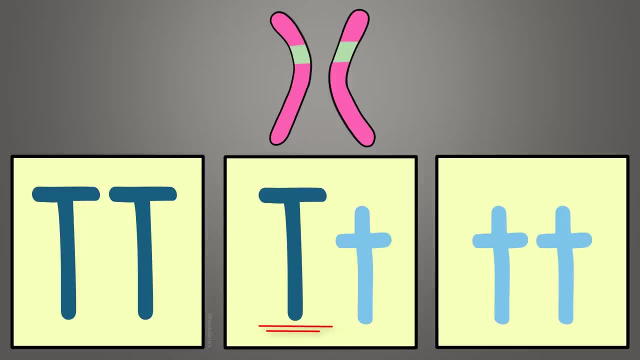 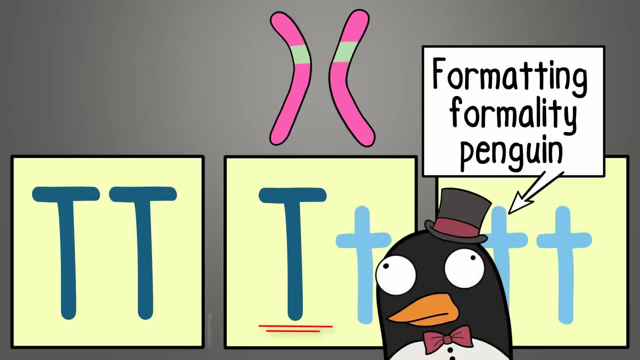 You'll notice, when writing genotypes I put the capital letters first. if it contains a capital letter, That's not because the order matters. it's a formatting formality that capitals are written first. It turns out that being able to taste PTC is a dominant trait. That means the phenotype. 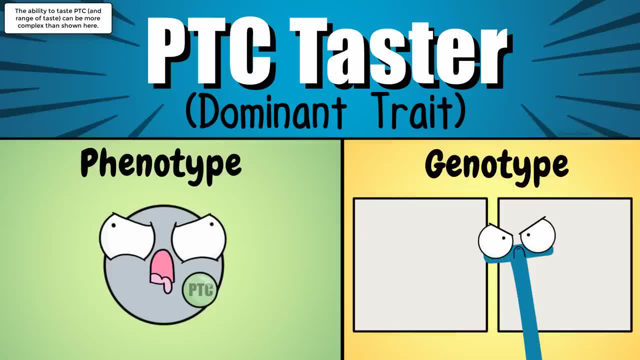 which is a PTC taster, is due to a genotype that includes at least one dominant allele. So which genotypes can taste PTC then? Well, big T, big T can. both of those alleles are dominant, So can big T, little t, because 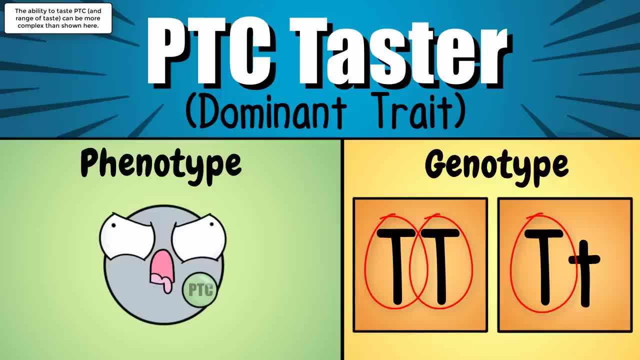 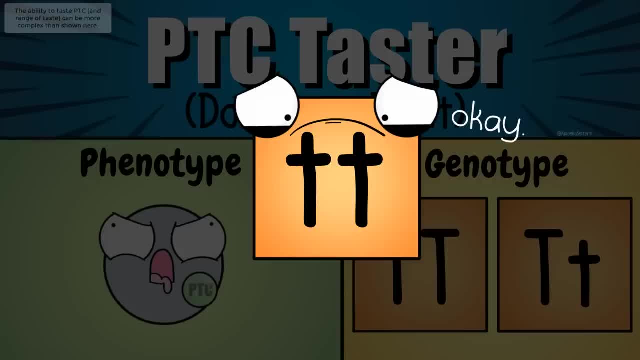 remember, it only takes the presence of a dominant allele to determine a phenotype. That's why, of one dominant allele, In fact, the only genotype in this simplified example to not be able to taste PTC would be little t, little t. So obviously, that is what I am. I am the little t, little t genotype which results. 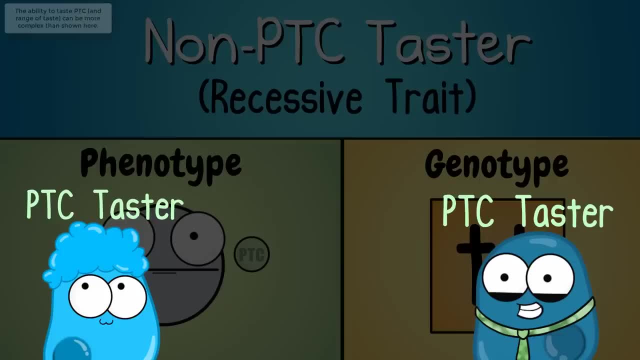 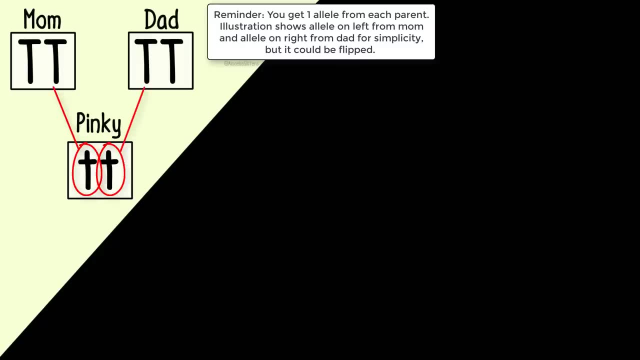 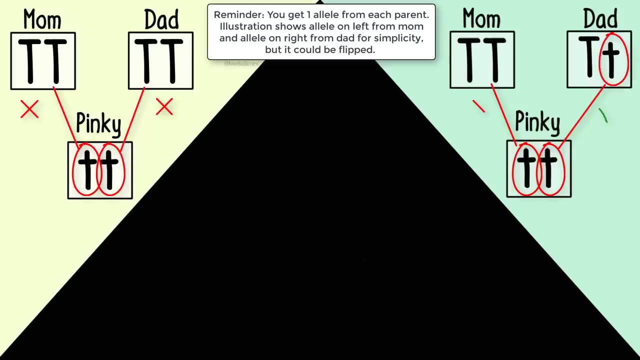 in my non-taster phenotype, But my parents can taste PTC, So what genotypes would they have to be? Well, if they were both big T, big T, that wouldn't be possible. If one was big T, big T and one was big T, little t, that still wouldn't be possible. Remember. 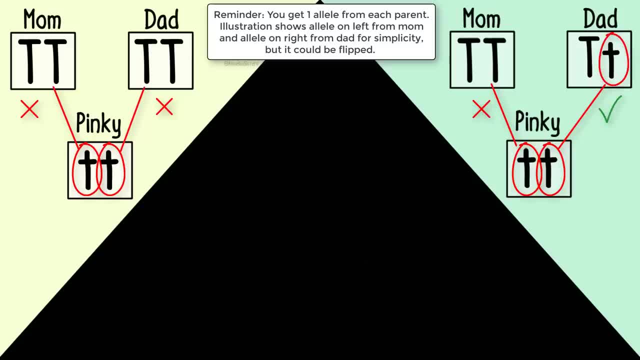 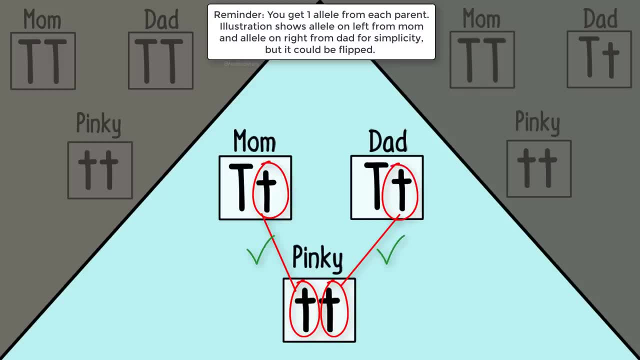 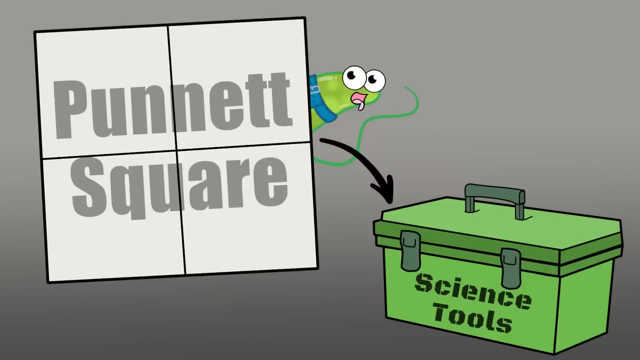 you have to get an allele, a form of a gene, from each parent. If my parents do taste PTC and I do not, then my parents have the genotype big T, little t and their phenotype is PTC. taster Punnett squares can be used to determine the probabilities of offspring having certain 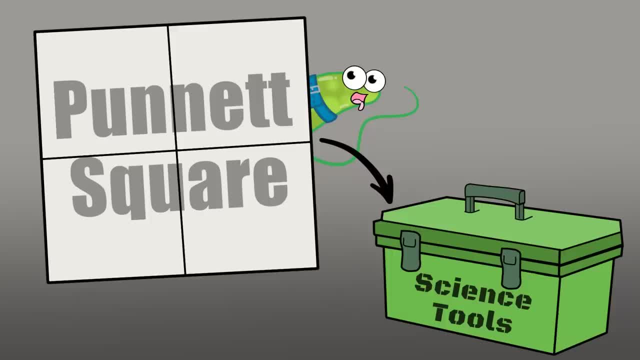 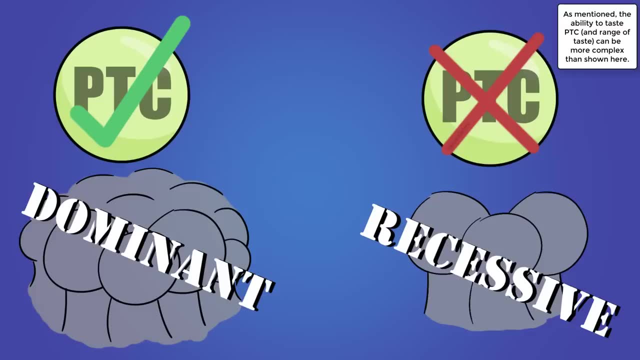 genotypes- which then can be used to determine their phenotypes. But punish that squares are for another Amoeba Sisters video. Before we end, one more thing to mention. In this example, the dominant trait of being able to taste. PTC is more common than the. 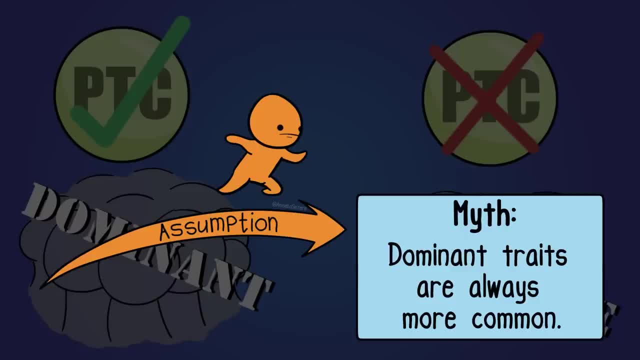 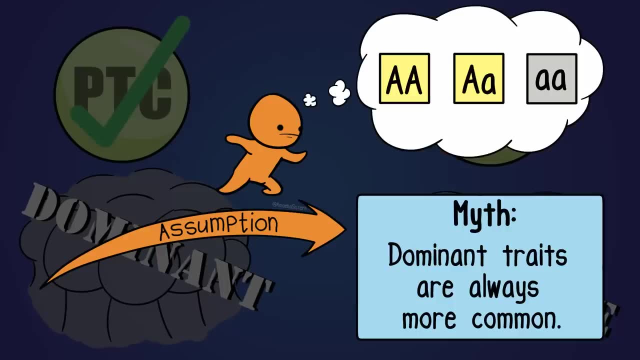 recessive trait of not being able to taste PTC, And one could jump to an assumption that dominant traits are more common, especially since it only takes the presence of one dominant allele to show up in the phenotype, At least in Mendelian inheritance. 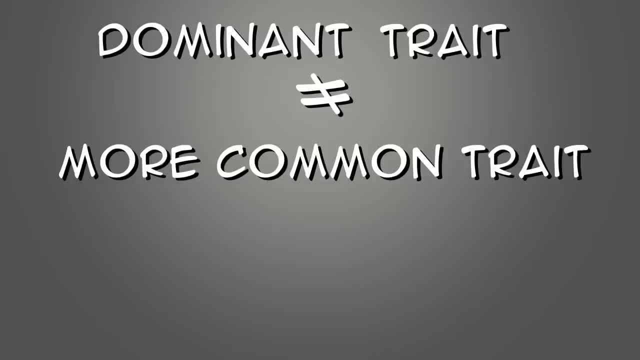 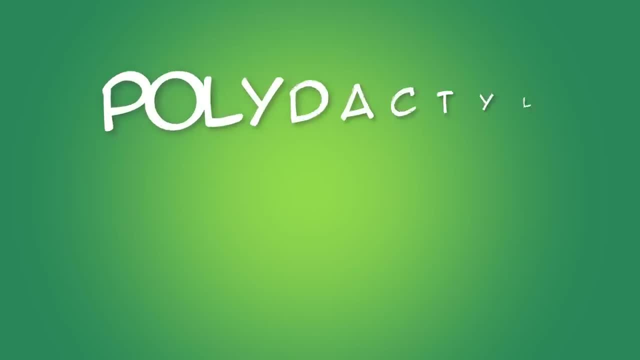 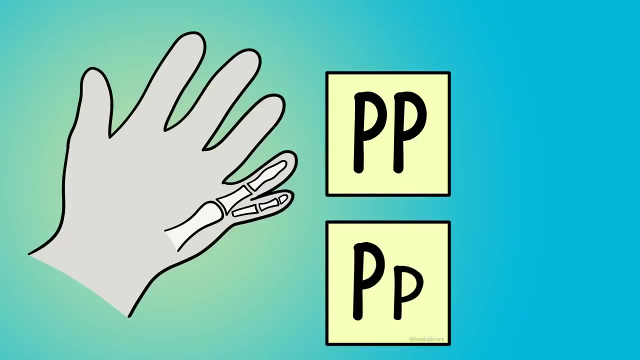 But the dominant trait is not always more common in a population, because it's possible that the dominant allele itself is more rare. That can be the case with some forms of polydactyly that is, being born with extra fingers. Some forms of polydactyly can be a dominant trait caused by the presence of at least one. 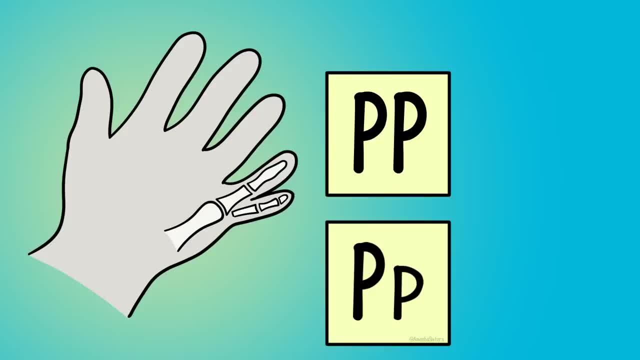 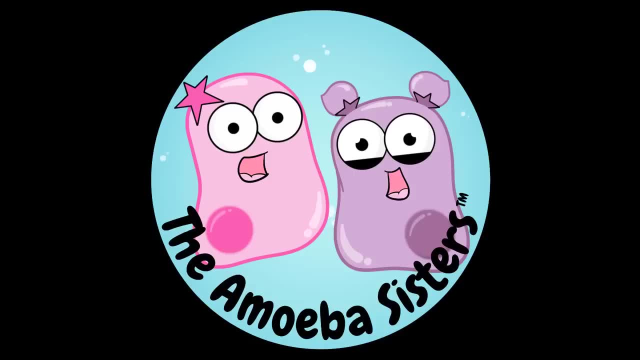 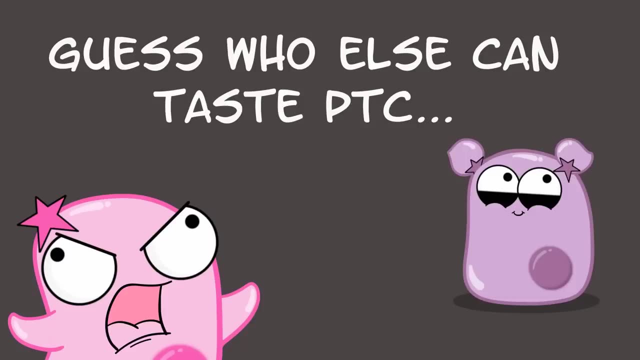 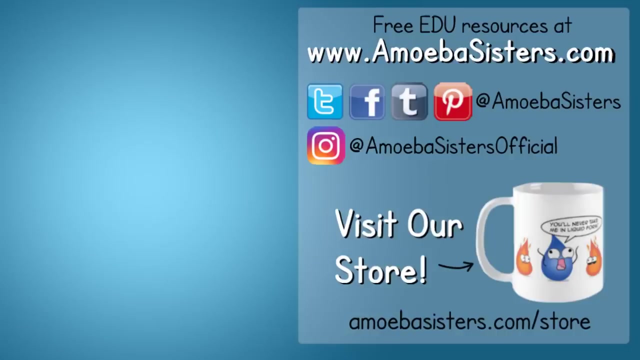 dominant allele. However, the dominant allele may not be as common in the population and the condition of having extra fingers is generally rare. Well, that's it for the Amoeba Sisters video. Thanks for watching and we remind you to stay curious.